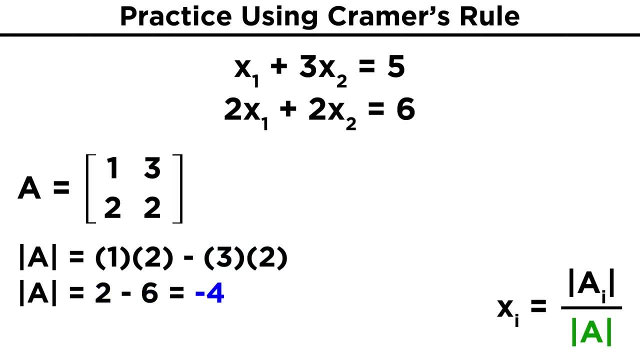 the bottom left. This gives us two minus six or negative four. Now let's talk about the matrix that goes on top. For the first variable, X one, we will have to replace the first column of the coefficient matrix with the constants five and six that we see on the right side of these equations. 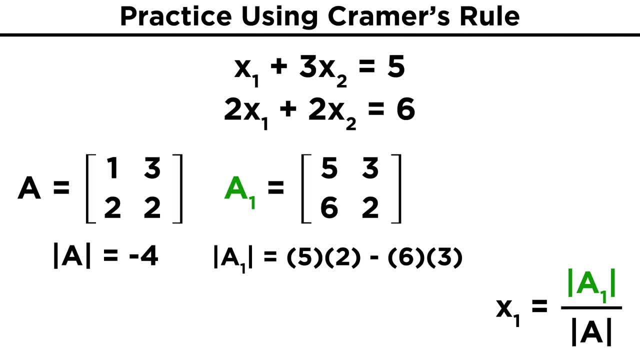 and then we will find the determinant of this new matrix. This will be five times two minus the quantity, six times three or ten minus eighteen, which is negative eight. Then, to solve for X one, we simply divide the determinant of the altered matrix by the. 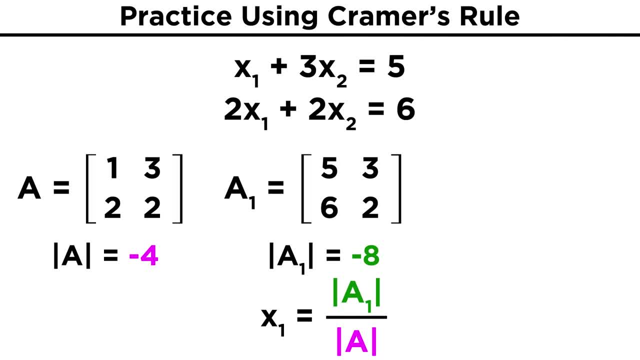 determinant of the coefficient matrix, which we already calculated, and negative eight divided by negative four gives us a value of two for X one. Now let's solve for the second variable, X two. To do this, it's almost the same thing. the only difference is that we will replace 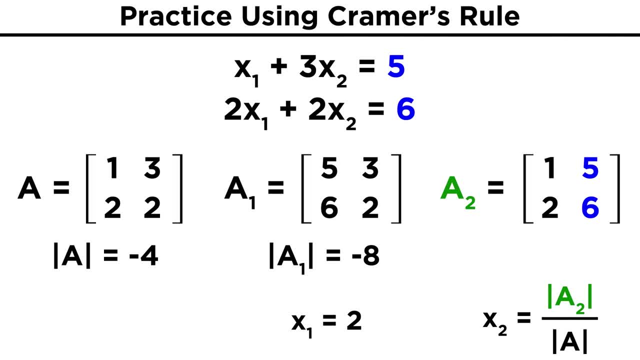 the second column of the coefficient matrix with five and six Rather than the first, because we are solving for the second variable. Now we can find the determinant of this matrix. This time we get one times six minus the quantity, two times five or six minus ten. 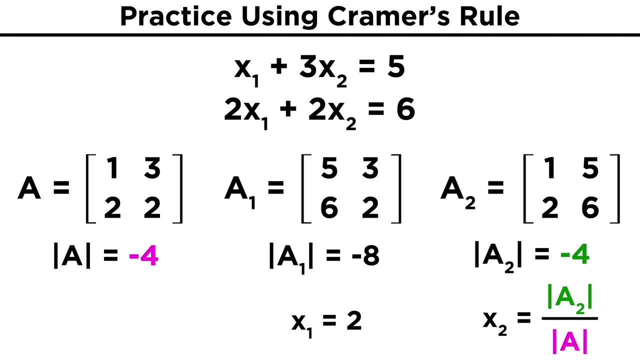 which is negative four. So we can take that and divide by negative four, just like we did for the first variable, because the determinant of the original coefficient matrix didn't change at all. And negative four divided by negative four gives us a value of one for X two. 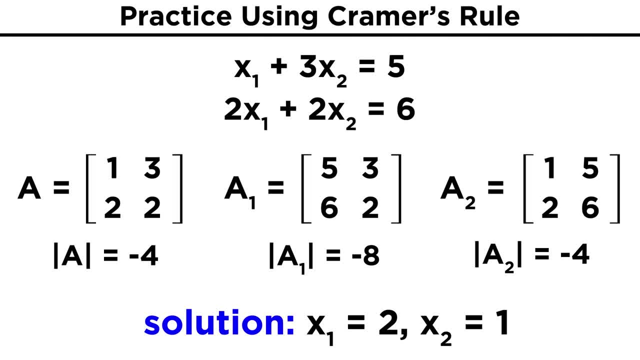 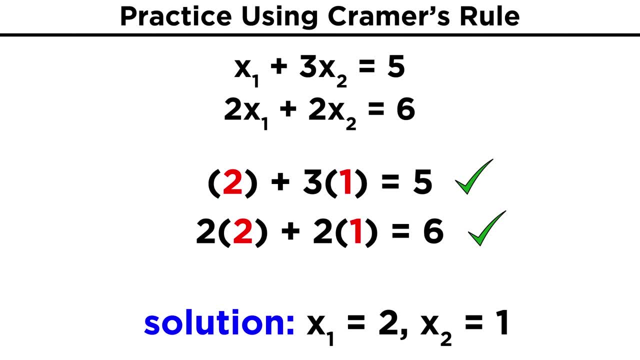 And there we have our solution for this system of equations: X one equals two and X two equals one. If we wish, we can plug these values into the original equation to verify that they work and, in turn, that this algorithm worked nicely. 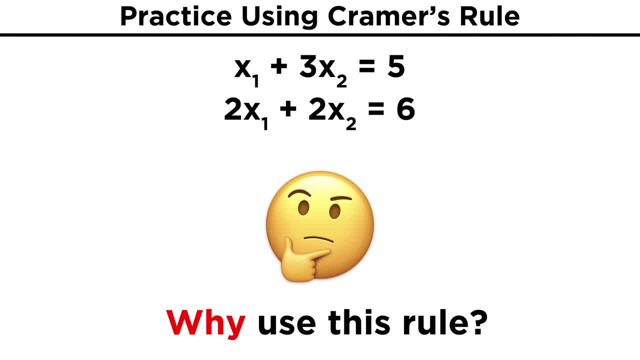 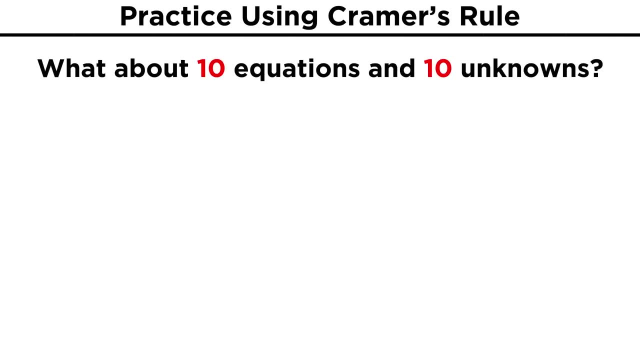 Now we might wonder why we would want to do this, Why we would want to use this, as it seems like a lot of work when we could have solved this very quickly by substitution or elimination. But the thing to remember is that systems of equations can get very complicated and 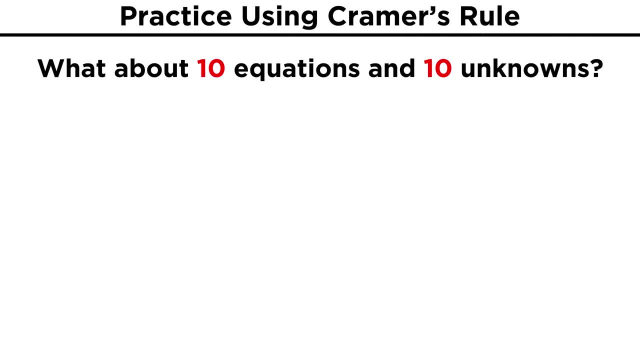 solving ten equations with ten variables won't seem so easy by previous methods. Cramer's rule is a simple algorithm that works precisely the same way for any number of equations With that same number of variables, So long as the system has a unique solution. 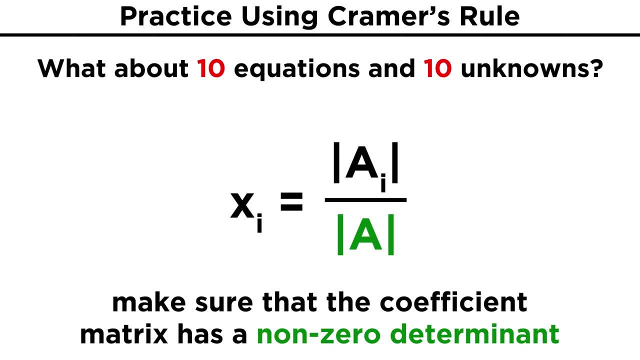 If the coefficient matrix has a determinant of zero, we will not be able to use this rule, as there is not one unique solution. But this is easy to spot, as we would need to divide by zero when solving for any variable, and of course that's not possible. 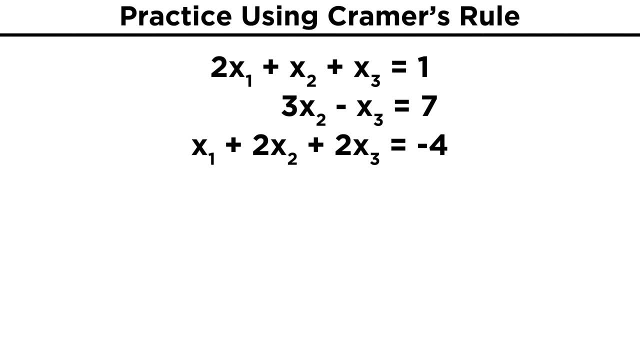 Now that we are warmed up, let's look at another example, this time with three equations. Let's look at the first example. Let's look at the first example. Let's look at the second example. There are three equations and three unknowns. 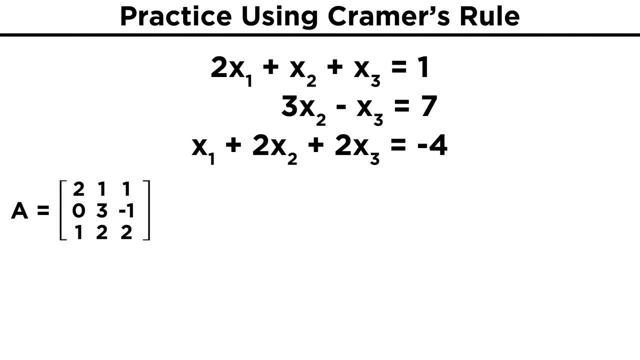 First, let's set up the coefficient matrix and find its determinant. If you need to practice finding the determinant of a three by three matrix, go back to that tutorial now. otherwise here we will just skip ahead to knowing that the answer is twelve. Now let's set up the three other matrices that will be involved in the rule replacing. 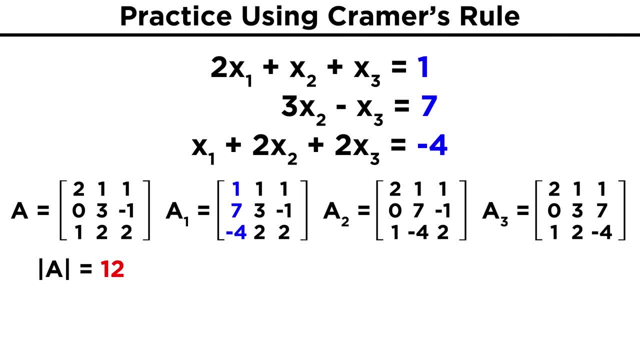 the first column with the constant term, And the first column will be a new one. constant terms will give us A1,, and this matrix has a determinant of 24.. Replacing the second column with the constant terms will give us A2,, and this matrix has 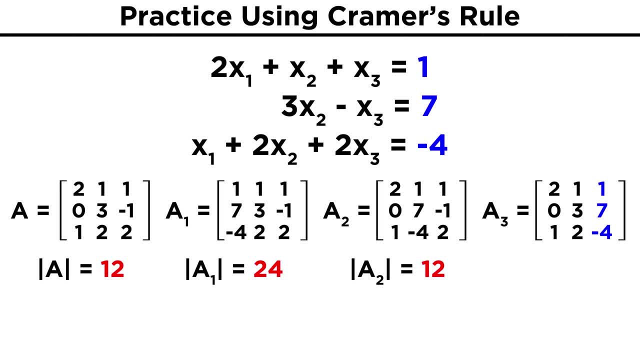 a determinant of 12.. Then we can do the same thing for the third column to get A3, which has a determinant of negative 48. With these determinants calculated, solving for the variables will be trivial. For X1, we take 24 and divide by 12 to get 2.. 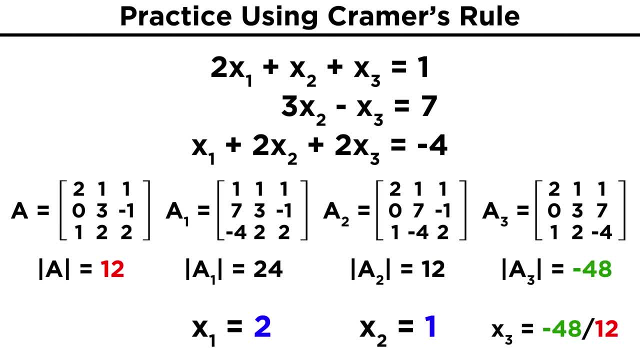 For X2,, 12 divided by 12 gives us 1.. And then for X3, negative 48 divided by 12 will give us negative 4.. And there is our solution to this system of equations. With this new and nifty trick under our belts, let's check comprehension.